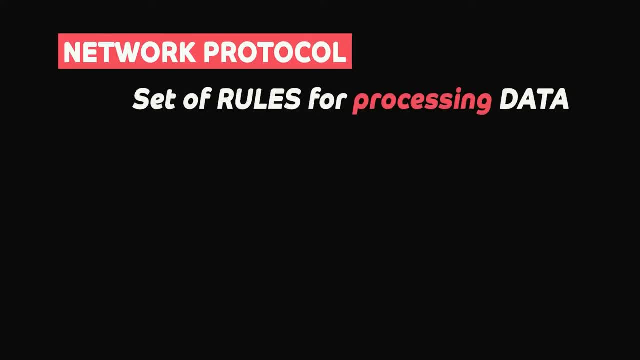 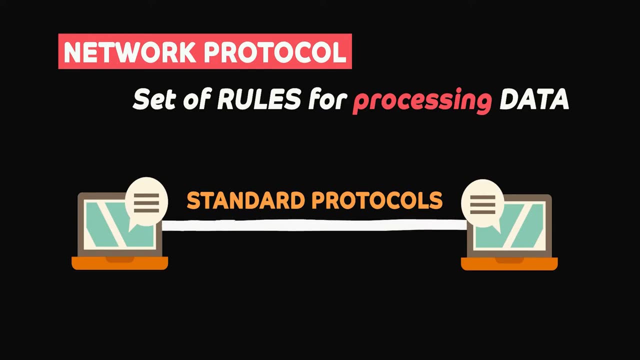 In networking, a protocol is a set of rules for formatting and processing data. Network protocols are like a common language for computers. Computers follow standard protocols to communicate and there are many, but for any system design interview, there are just three protocols 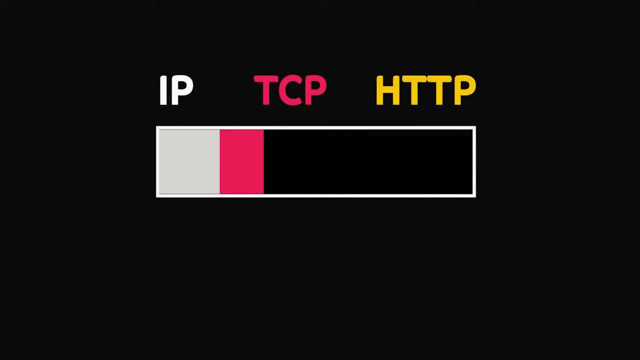 you need to know. IP, TCP and HTTP. When a machine sends data to another machine, it is sent in the form of IP packet. Think of IP packets as fundamental unit of data stored in bytes and two main sections here. IP header and IP version. IP header contains information about the packet such as source IP address, the destination IP, address the packet needs to go to and the packet size. The IP version could be IPV4 and IPV6 etc. The rest of the IP packet is data. This is 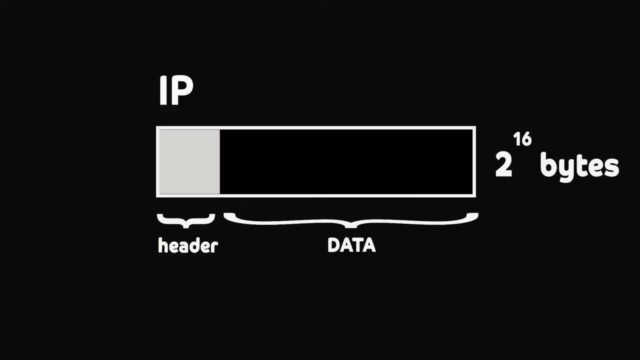 where the information one machine is trying to send to another machine is stored. The size of the IP packet is however limited, typically around 0.065MB to be precise. So if you're trying to send data to a computer, the packet size is around 0.065MB. standing on a computer And this is just fine. If you weight it around 40.1MB, screws it around, you don't need to do it. 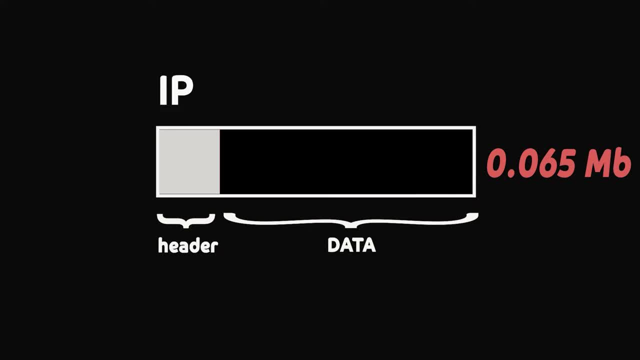 send an email, let's say with some pictures attached, it needs to fit into multiple IP packets. Now when you send all these IP packets, you must guarantee the order in which they are being sent, so that the receiver gets the data in correct structure and take care of any lost 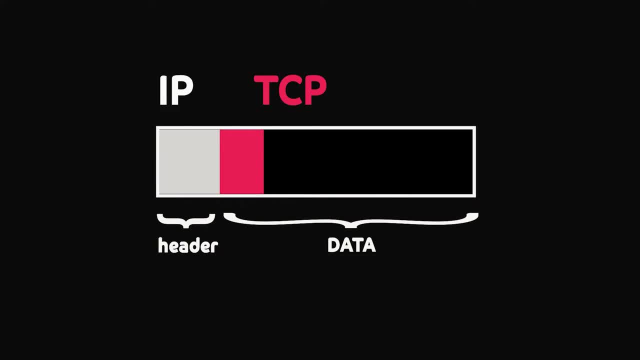 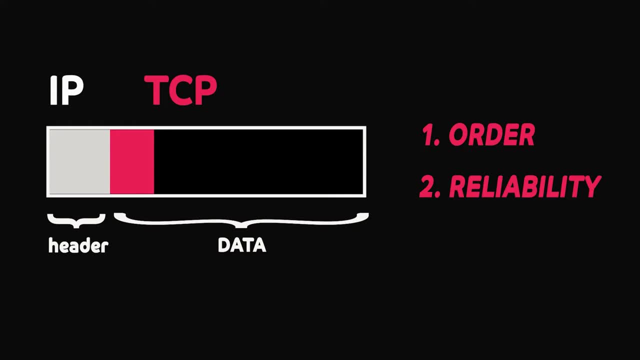 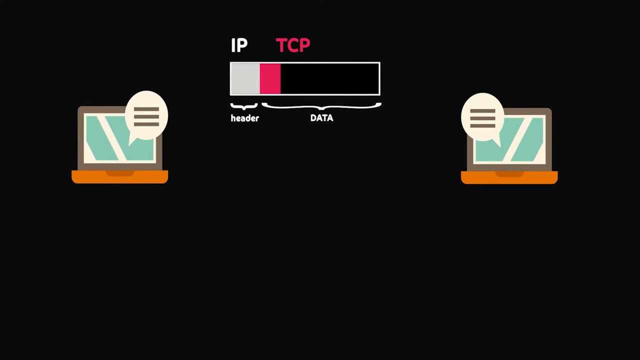 packets. This is where TCP comes into play, which builds on top of IP protocol. It pretty much guarantees two things. The IP packets are sent in an ordered way, and all packets gets received by the destination machine without being damaged. TCP is virtually used in all web application as it allows us to send long pieces of data which IP cannot do it on its own. To stitch together all the IP packets, each IP packet will have a TCP header in its data section. So when a client machine such as browser wants to communicate with the Amazon website servers, it first needs to create a TCP connection, and this process of initially setting up the connection is known as 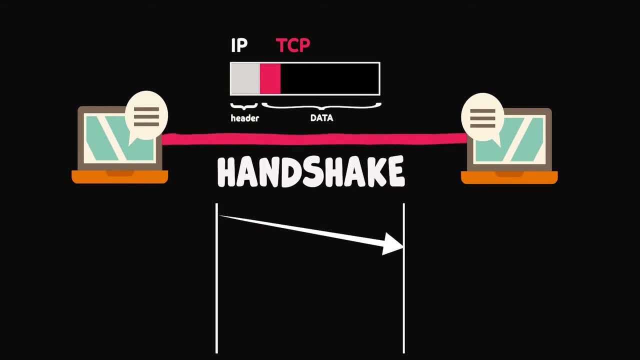 handshake. In handshake process, a machine usually sends packets to servers, and the server is saying, hey, I want to connect with you. And the server machine responds saying, 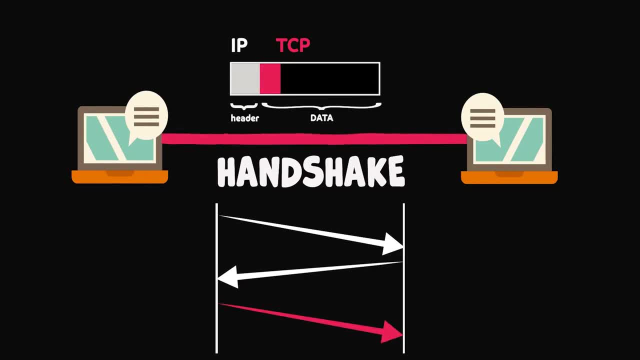 okay, we can connect. The client responds saying, okay, connected. The TCP connection can be terminated by either of the machines. For example, you closing the browser. And if any machine takes more than a fixed amount of time, the connection can time out, causing TCP connections to terminate.